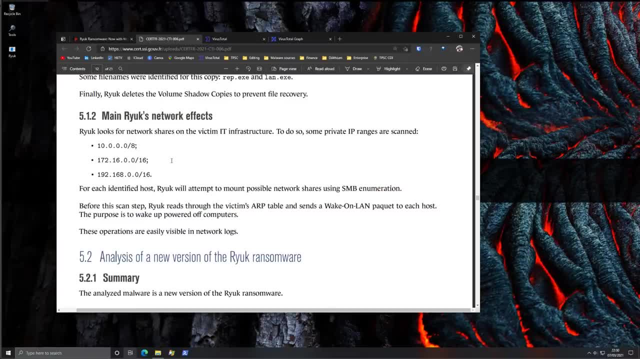 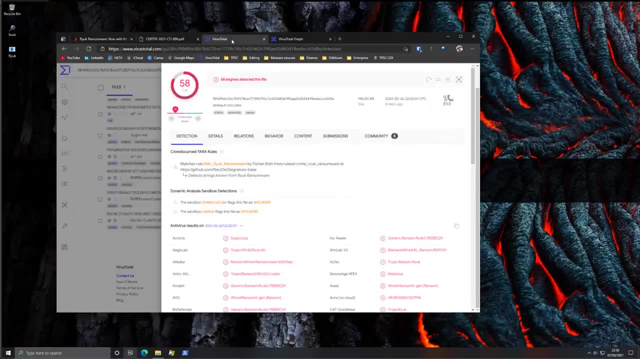 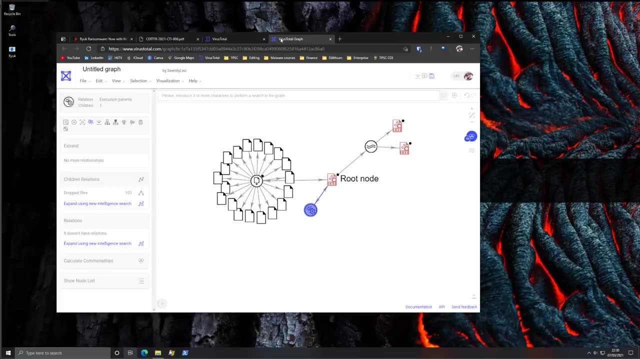 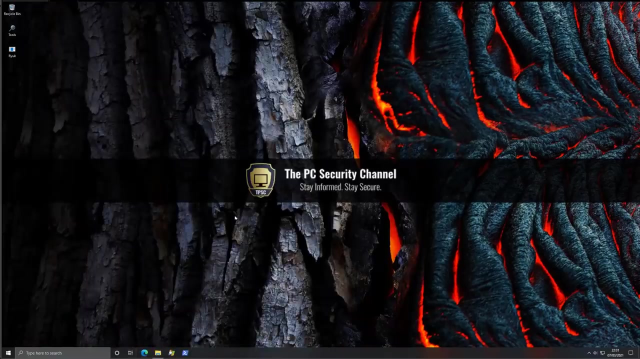 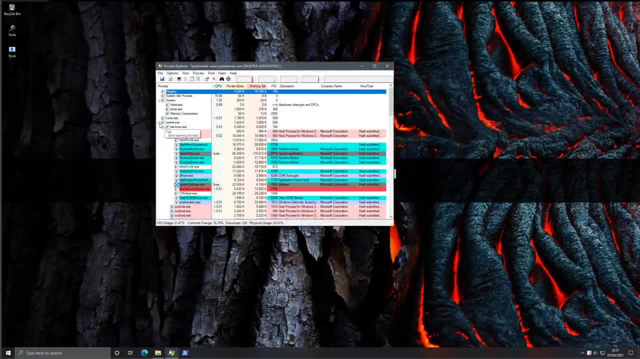 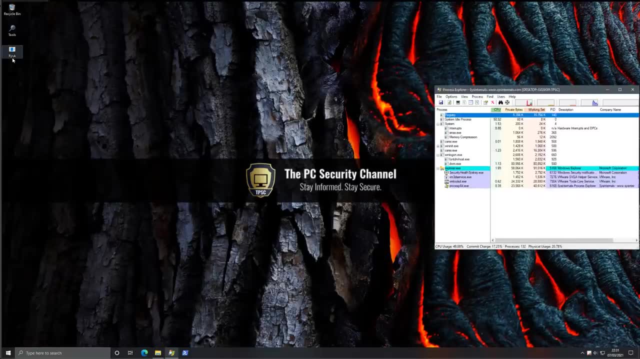 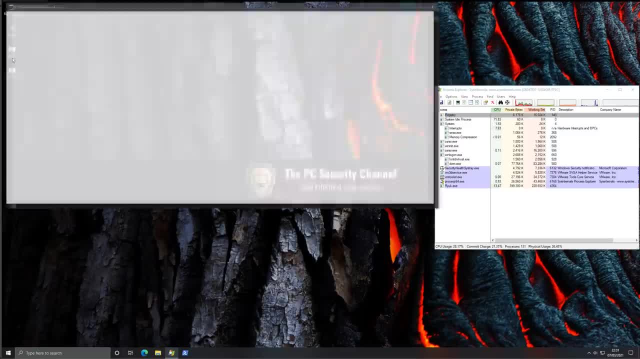 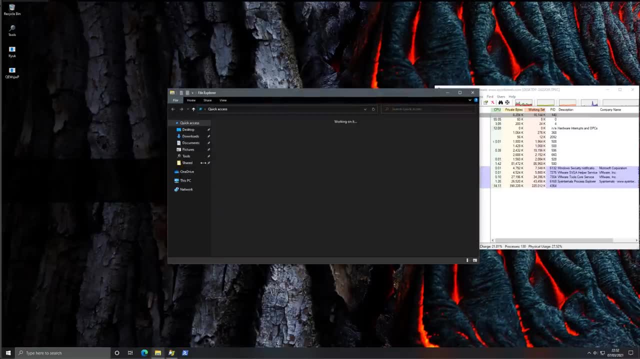 Within seconds, the subprocess terminates and by now, as we will see, our network location is probably already encrypted, even though we don't, you know, start to see things on the desktop until a few seconds. So, if we look at our network location, everything is already encrypted with the 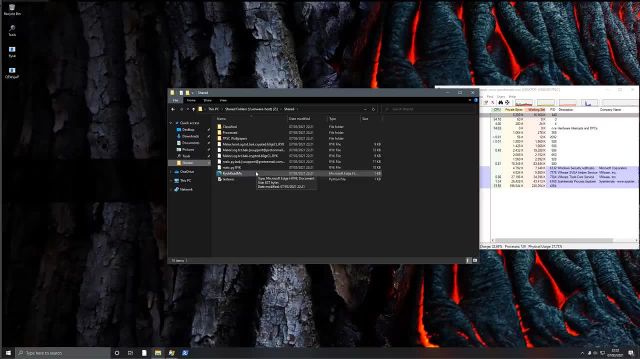 Ryuk extension. We've also got the Ryuk readme, and after some time we start seeing pop-ups like: your files are waiting to be burned to disk, and then we're going to see the readme on the desktop, as well as our documents and pictures being encrypted- Now for almost all variants of Ryuk. 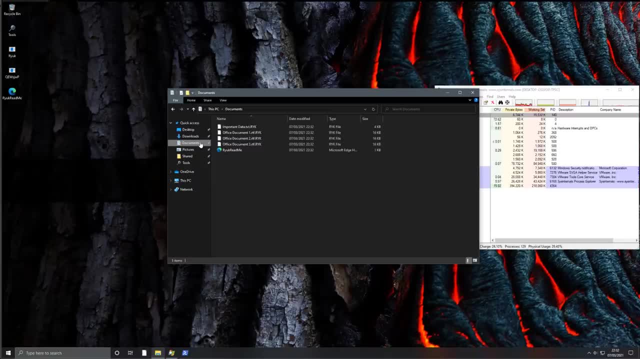 you're not going to be able to recover your files unless you have existing backups, and that's because the encryption process is quite secure. There are no obvious flaws that can be broken into unless you either have a partially working key, something of that sort, but without any help from. 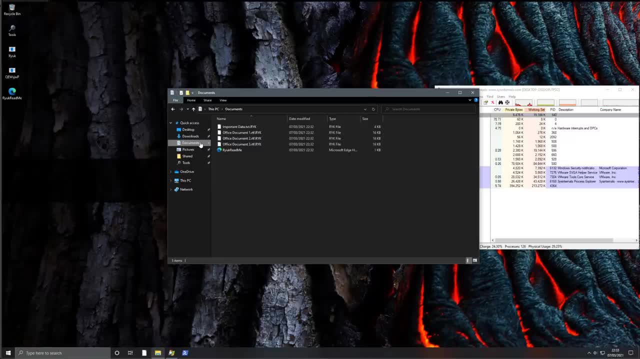 the attacker. So if you have a partially working key, you can't recover your files. unless you have hackers, It's often impossible to recover your data. Our pictures, as you can see, are encrypted as well. but again, the key thing to note here is it's going to attack the shared locations first. 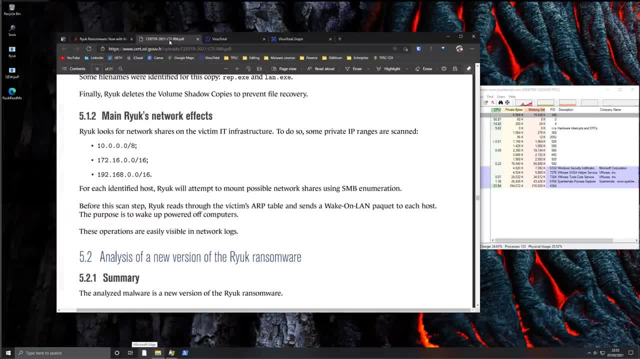 It's going to navigate the network, traverse through the range of IPs and then work its way backwards to the host system. In this case we just have one network. drive was encrypted in a flash, but in the case of an actual organization it could take several hours. 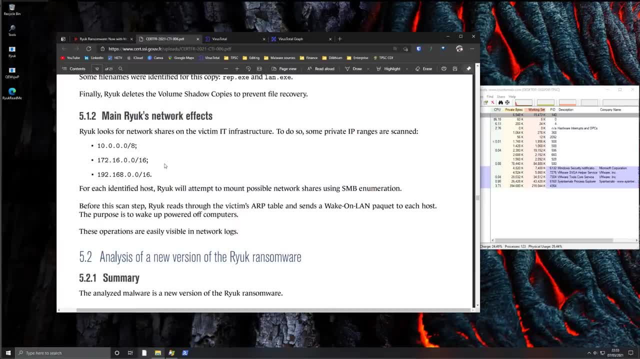 and that is why it's important to examine your network infrastructure and make sure your network drives are adequately protected, because it's not going to be easy to narrow down the system that's been compromised that's actually executing the ransomware if your network drives start. 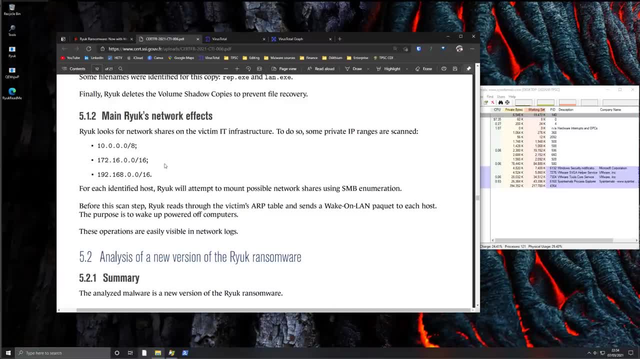 getting encrypted. Now, if you're thinking that our network locations are not necessarily always active, that's not going to save you because Ryuk is going to read through the ARP table and send a wake-on message to the ARP table and that's going to save you a lot of time. So if you're thinking 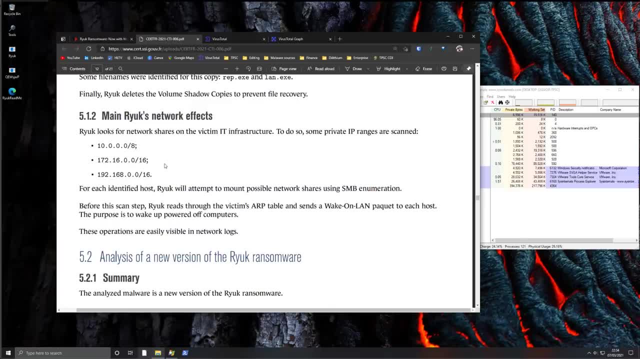 that our network locations are not necessarily active. that's going to save you a lot of time. So if you're thinking that our network locations are not necessarily active, that's going to save you a lot of time. So if you're thinking a LAN packet to each host. So if you see something like this in the network logs, act immediately. 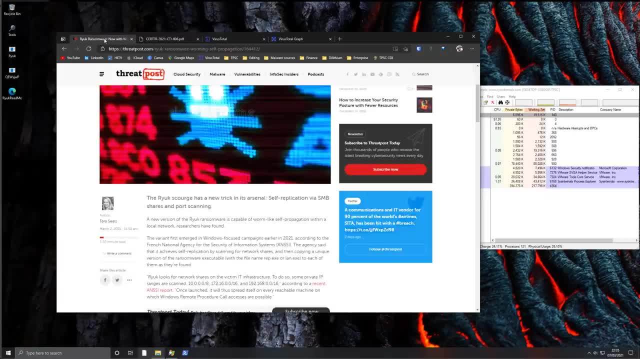 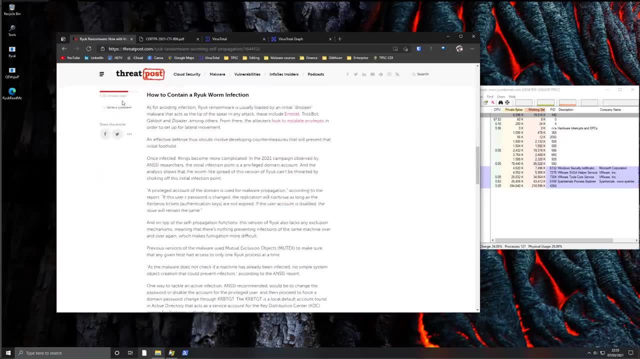 It is also worth noting that Ryuk is one of the most persistent of ransomware. They're actually spread via many different methods, including Imhotep, Trickbot Zloader and other such exploits. Imhotep was recently shut down by enforcement agencies, but some of the other ones are still. 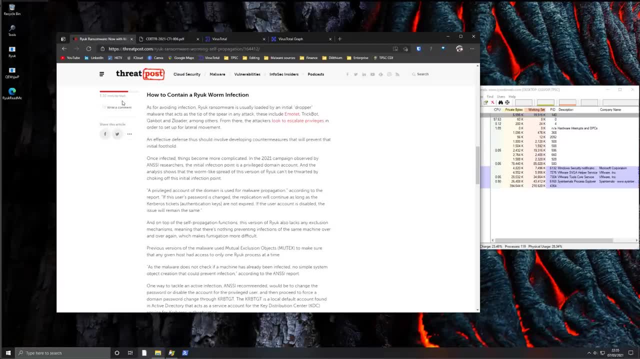 active. In a lot of cases the attack is going to be only in the network logs and that's going to are targeted and quite successful. I suspect this is one of the top grossing ransomware in terms of the money brought in and we've had a lot of threats that come and go. they have their heyday. 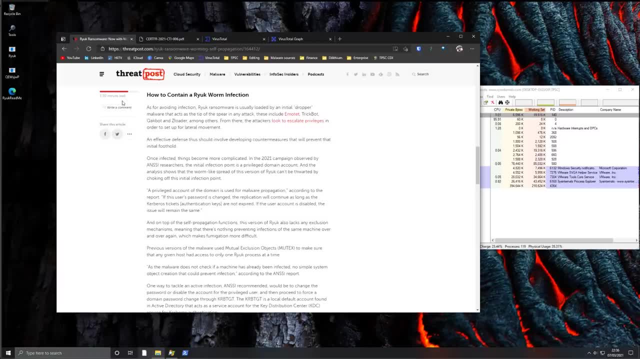 and then they're shut down or the ransomware authors just decide: well, we've had enough. we don't want to keep going at this game, but Ryuk is one of the most persistent threats. I believe most of the threat actors are based in Russia and even after two years we're seeing new variants. we're 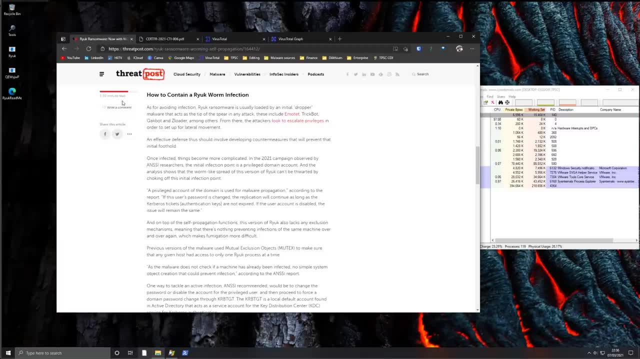 seeing a lot of activity associated with this threat. this is partly why we design our test scenarios for testing AV products, mostly modeling this kind of ransomware behavior in terms of attacking shared locations, starting from the host and then encrypting files on other systems, because that's just a devastating model that Ryuk has used to full effect and other infamous ransomware do as, 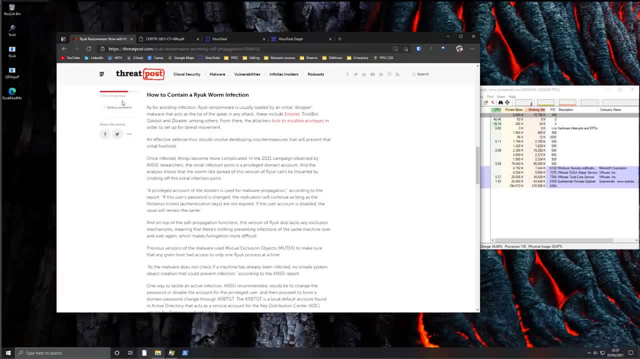 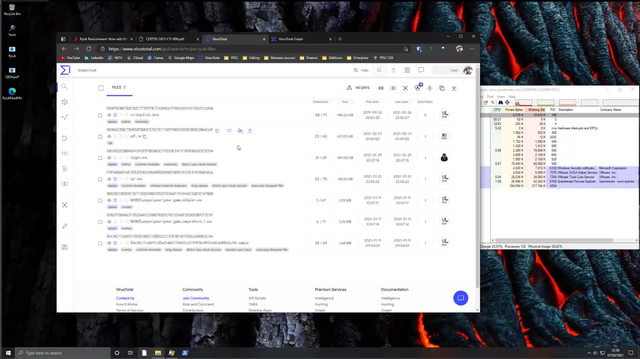 well. by the way, if you're a business and you'd like to figure out how you would fare in the event of such an attack and test your own security systems, feel free to contact us at the pcsecuritychannelcom. now. some variants of Ryuk will also avoid sandboxes. they will not run in an external. 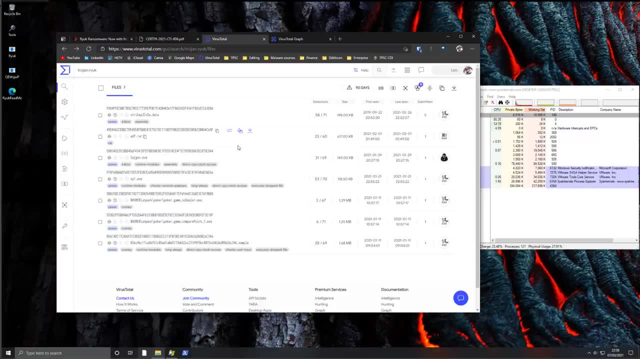 environment, and that prevents a lot of the sandbox based detection systems that are in place these days for certain AVs. they will perform a lookup on the cloud. if the file is unknown, they will run it in their own sandbox and use that data to quickly evaluate the data and test your own. 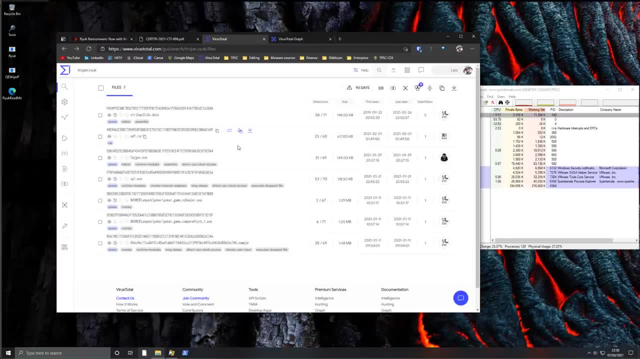 system, if it's malware or not, and if the malware just avoids their sandbox, doesn't perform anything malicious there, well, the AV is clueless and will let the file continue executing on your system, where it will perform the malicious behavior. this is also partly why I'm not super impressed with 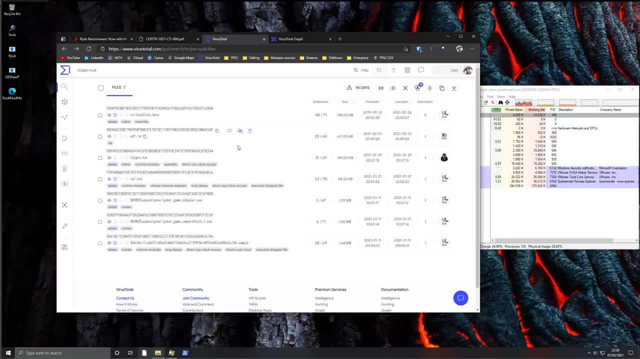 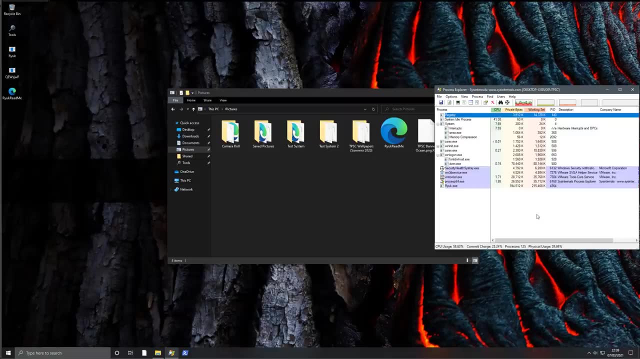 systems that rely entirely on the cloud, because, at the end of the day, the action happens on your system. it is on your system that the process is going to execute. it is on your system that the files will be loaded into the CPU registers. it is on your system that the files will get encrypted. 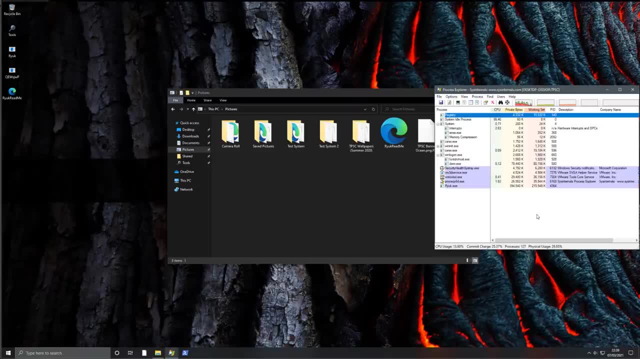 so it's crucial to have defenses there that are not dependent on external systems, necessarily, but anyway, I hope you enjoyed this quick overview of Ryuk. it is a pretty infamous ransomware and if you'd like to learn more about how you can prevent ransomware from encrypting your system, what you 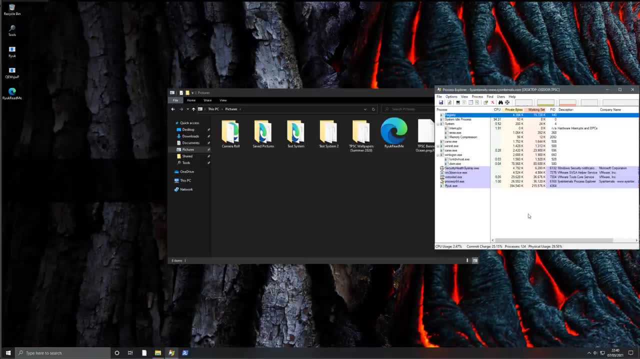 can do if you are encrypted and are looking for options for decryption. we've made dedicated videos about that in the description below, and if you'd like to learn more about how you can prevent ransomware from getting encrypted and decrypting your system, you can check out the video called 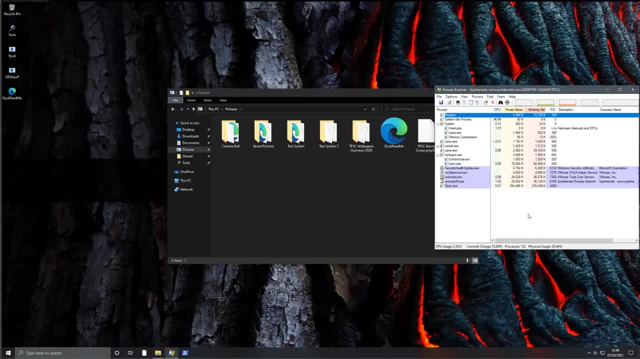 dealing with a ransomware attack and decrypting ransomware. make sure you like and share the video if you found it useful. we're now one of the largest cyber security channels on youtube and there's a lot of exciting content and announcements coming up, so join us. we also. 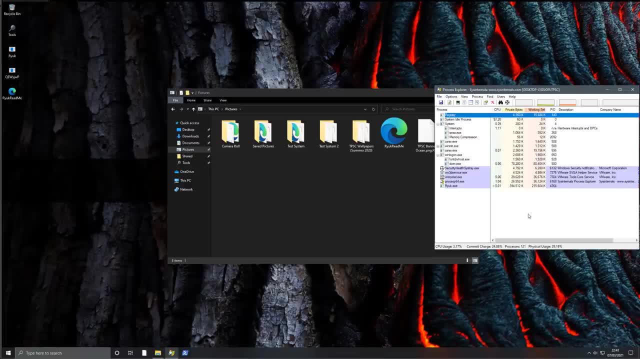 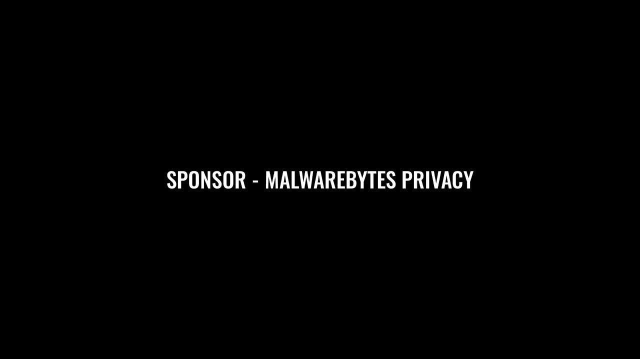 have a discord link in the description, in case you want to post video ideas, join the community, have any questions. I check that every day so you can reach me there. and now a word from our sponsors. many of you may be familiar with the name Malwarebytes. 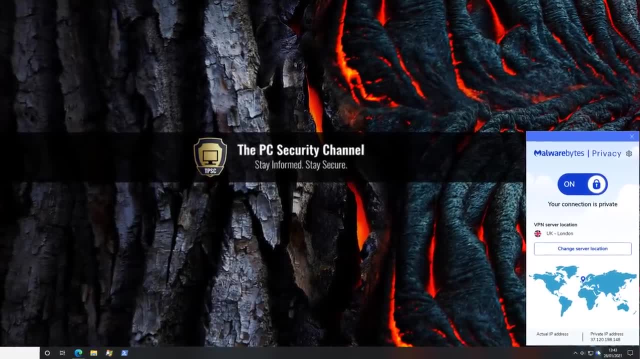 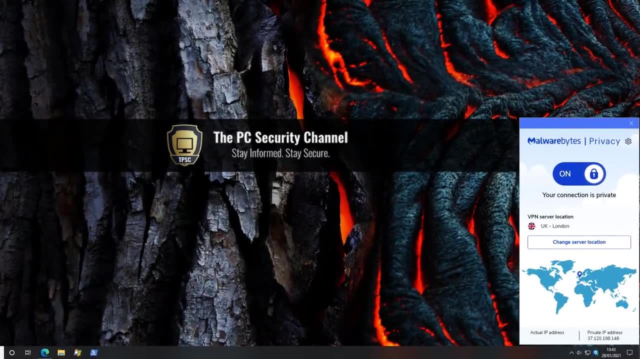 when it comes to anti-malware, but they have recently launched a brand new VPN service called Malwarebytes privacy. I've been running and testing this for the last two weeks and one of the most amazing things I've noticed is the speeds and consistency, especially in servers in the United. 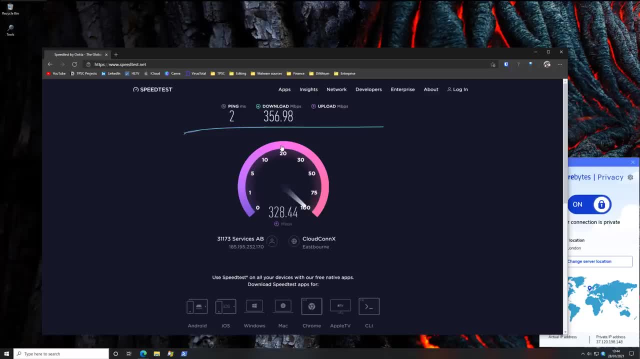 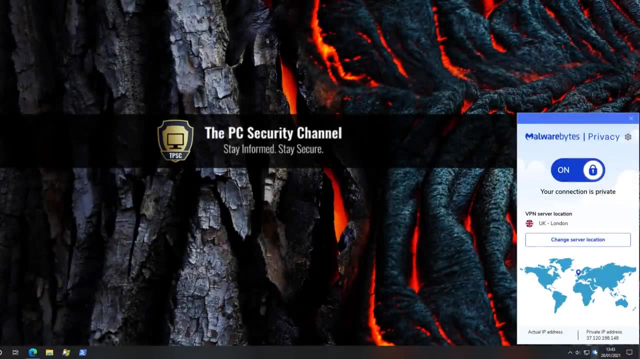 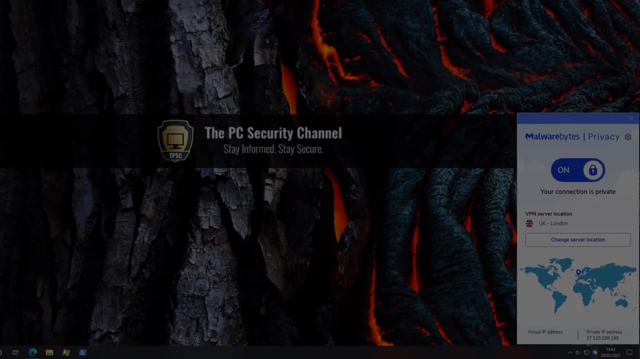 States and Europe. in some cases I've noticed it to be faster than some of the mainstream VPN providers. and this is a VPN service that focuses on being a VPN. they don't offer any cyber security protection with it, which means no tracking at all. they don't store any logs. the cyber security 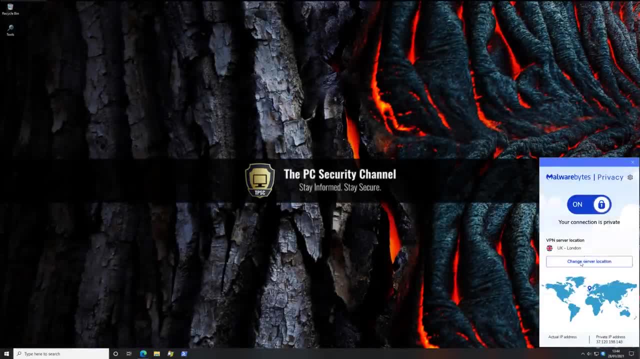 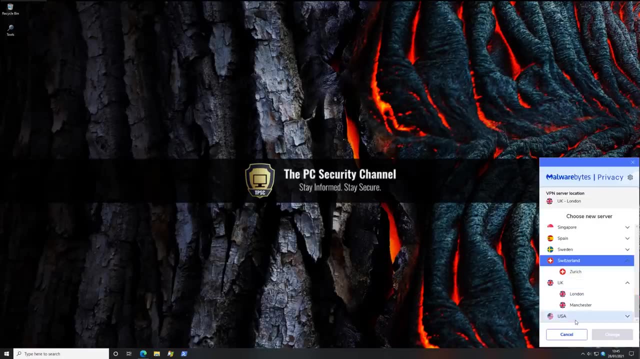 component is offered as an entirely separate browser extension. you can connect to servers in any country and once you do so, it's going to remember your choice and auto connect to you next time. so it's a full featured VPN. they do have a combined offer where you can get it at a discount. 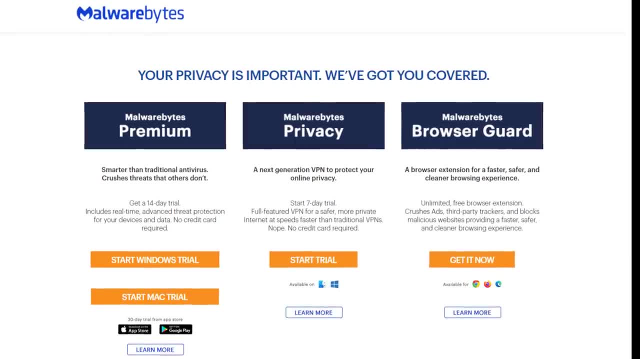 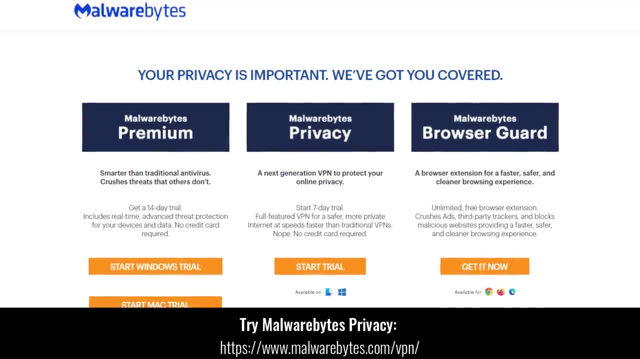 so if you are already planning on getting Malwarebytes anti-malware or already use it, it might be a really good deal for you. so show them some love for sponsoring the pc security channel. check out Malwarebytes privacy. link will be on screen and in the description. 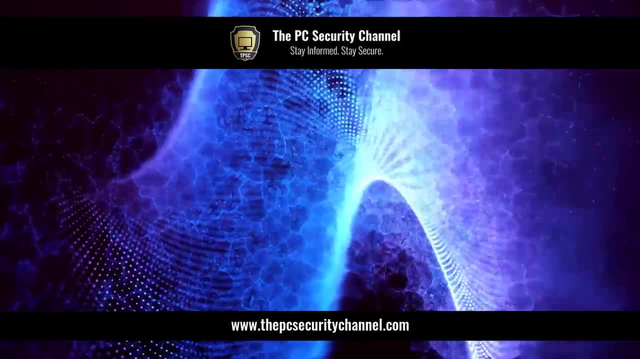 once again, thank you so much for watching and, as always, stay informed, stay secure. 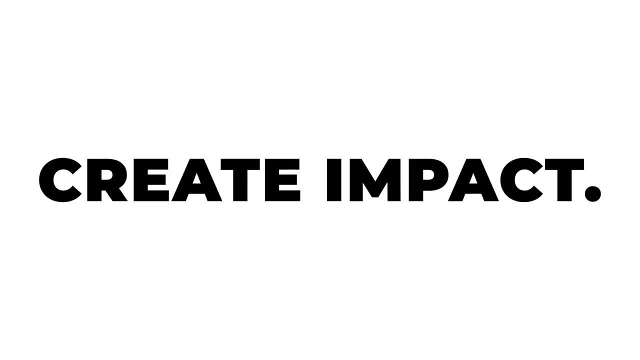 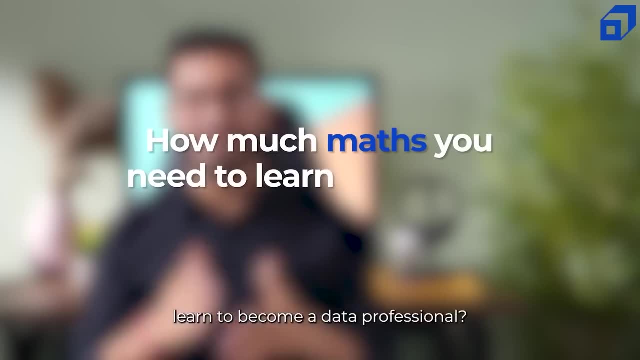 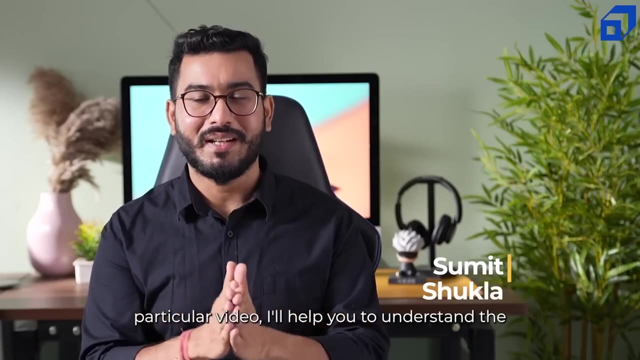 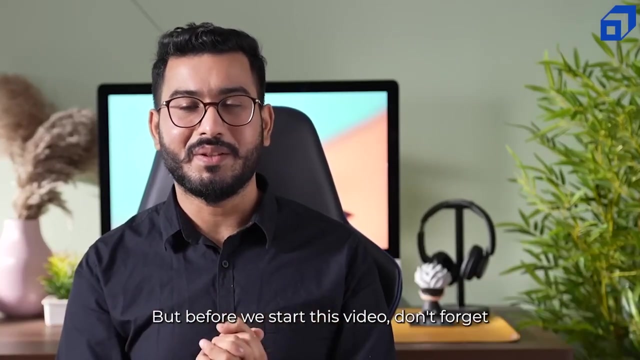 Hello, my name is Sumit Shukla and in this particular video I'll help you to understand the various topics you need to be aware about before you can become a data professional. But before we start this video, don't forget to check out Scalar's free masterclass on.